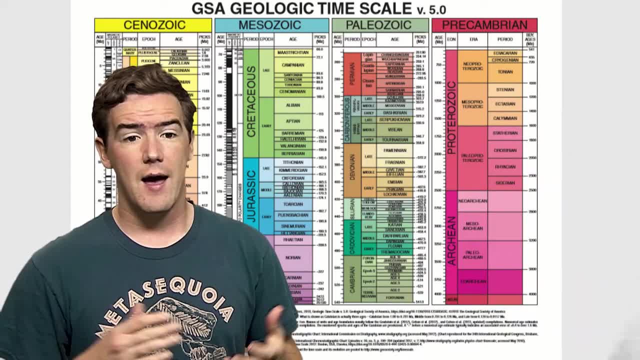 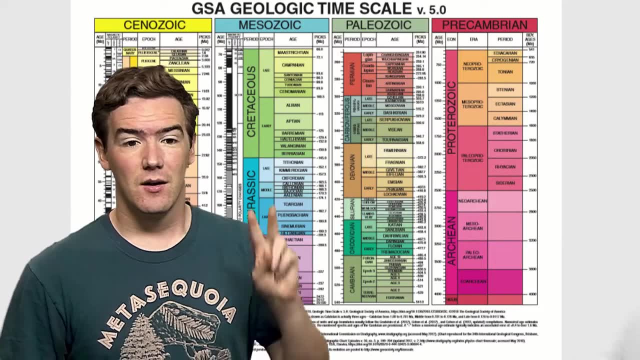 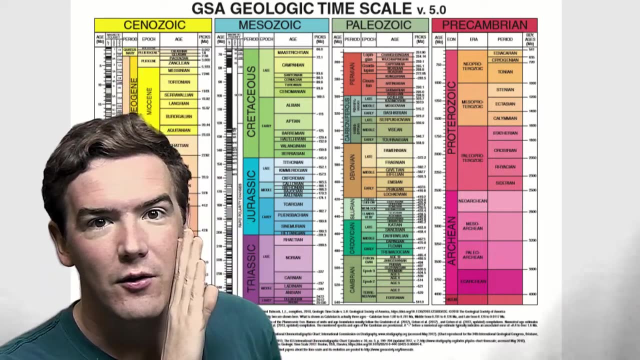 And this is unlike political divisions of land where you can have multiple things with the same name. For example, Washington. You can have the state of Washington, Washington DC, or multiple Washington counties throughout different states. But we all know there is only one Washington 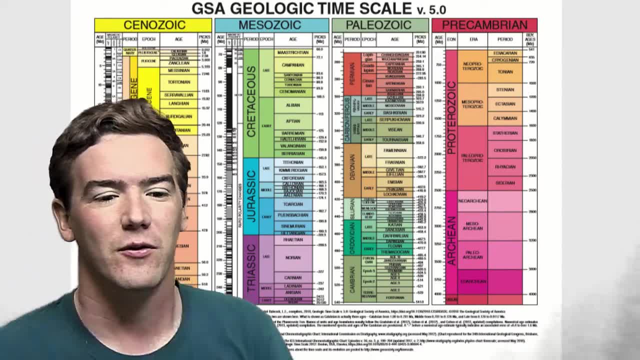 that is the state of Washington. Hashtag West Coast Best Coast. So how do we organize time? 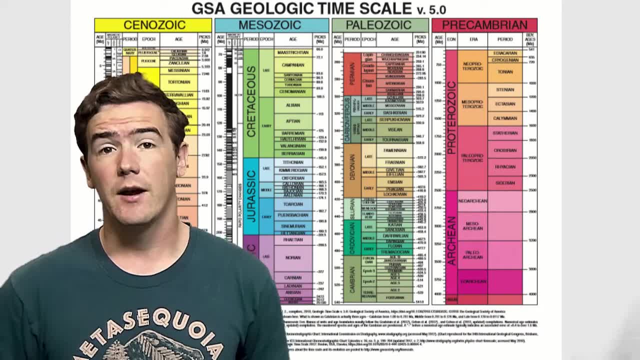 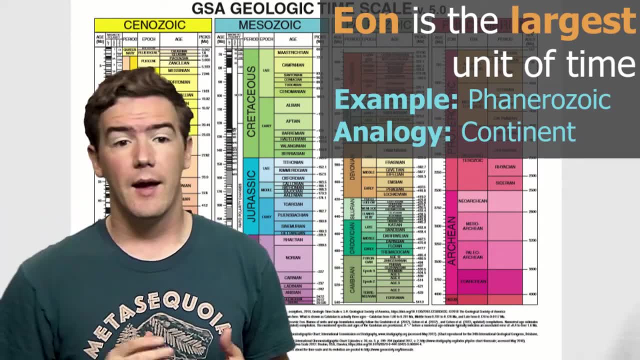 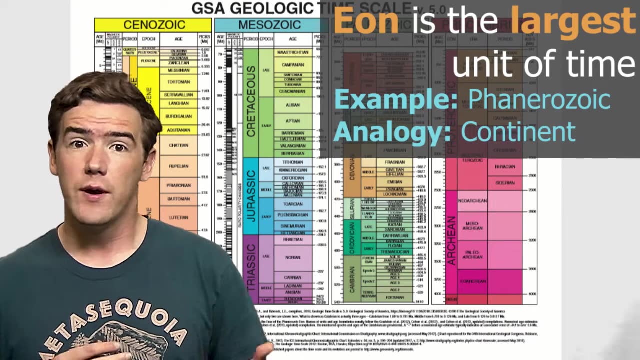 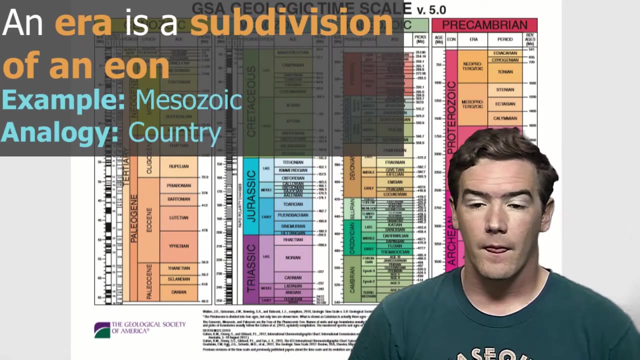 Our largest unit of time is called an eon, and currently we live in the Phanerozoic Eon. The Phanerozoic Eon is where we have the greatest diversity of life, and is usually the eon that most paleontologists study. If we are continuing our land analogy, we can think of an eon as a continent. Now within the Phanerozoic Eon, we have three eras. They are the Paleozoic, the Mesozoic, and the Cenozoic. 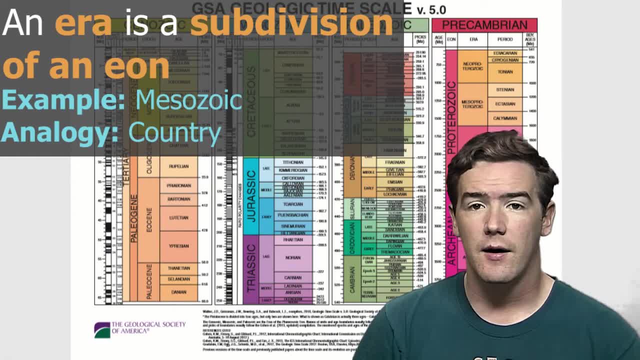 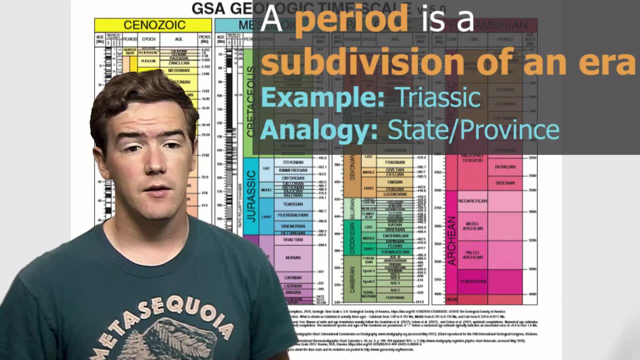 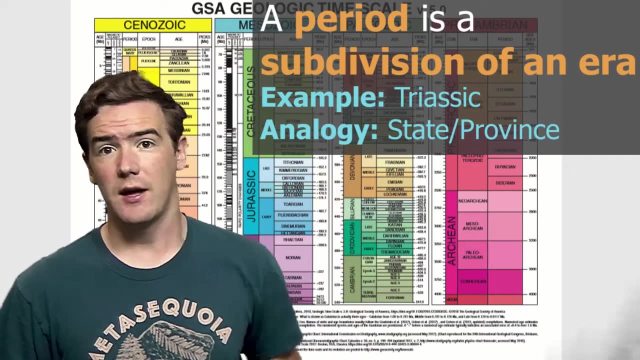 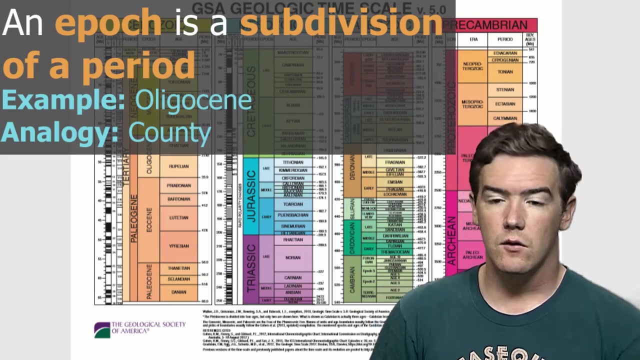 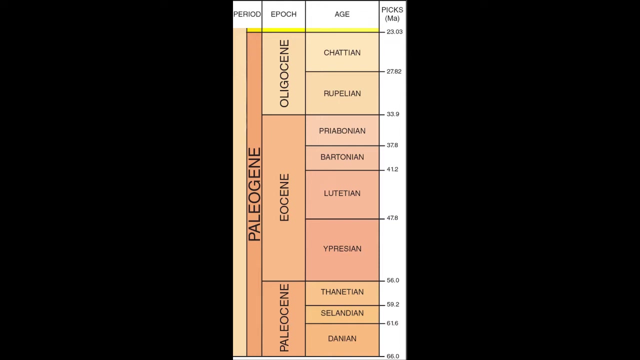 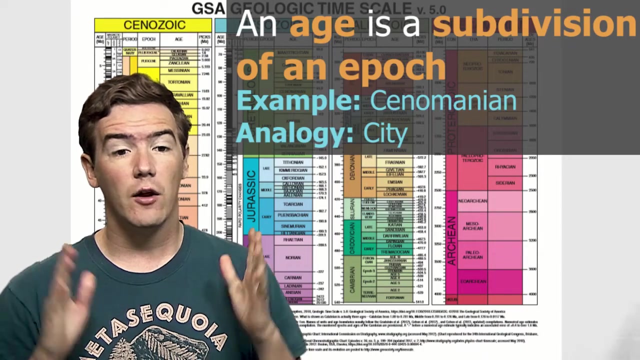 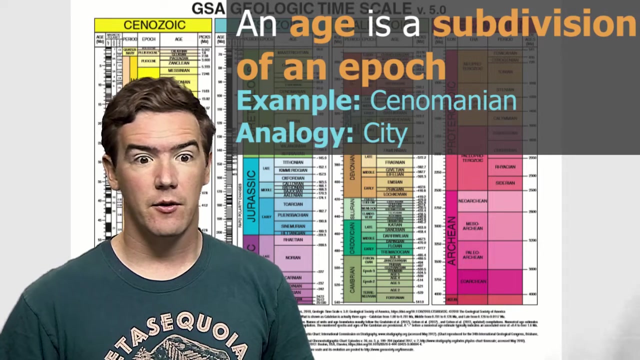 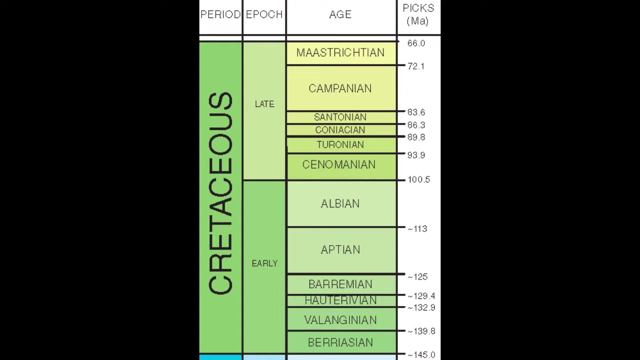 And further continuing our analogy, we can think of an era as a country. Within each era, we have multiple periods, and we can think of these as states or provinces. For example, in the Mesozoic era, we have the famous Triassic, Jurassic, and Cretaceous periods. Up next, we have epochs, and we can think of epochs like counties. Using the Paleogene as an example, which is a period in the Cenozoic era, we have the epochs Paleocene, Eocene, and Oligocene. And finally, our smallest unit of time is called an age, and we can think of an age like a city. So using the Late Cretaceous as an example of an epoch, and as a side note, Cretaceous is the period, but Early Cretaceous is an epoch, and the division of a Late Cretaceous is also an epoch. We have the 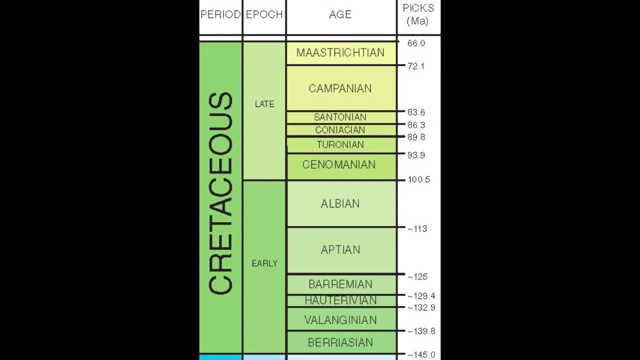 ages Sinomanian, Tironian, canuasian, santonian, keftian, and mastrictkan. 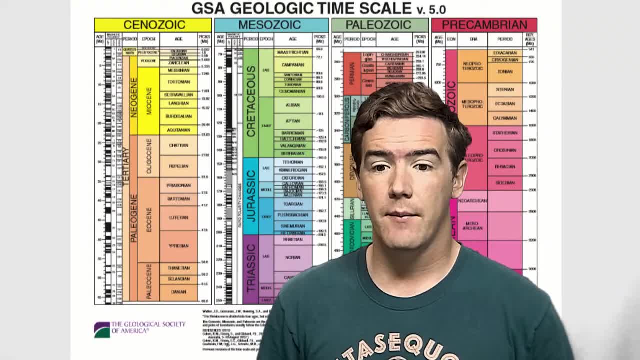 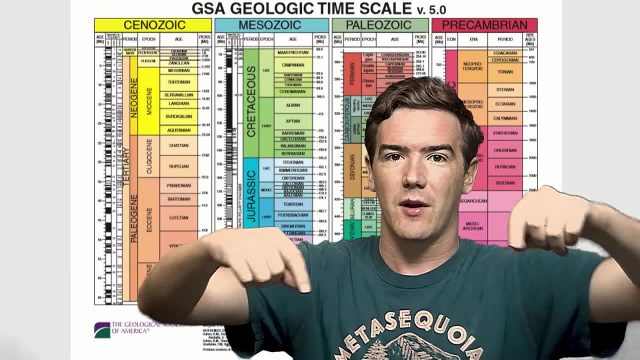 If you'd like a complete overview of geologic time and major events that happen within each period, you can make that suggestion for us in the comments below.